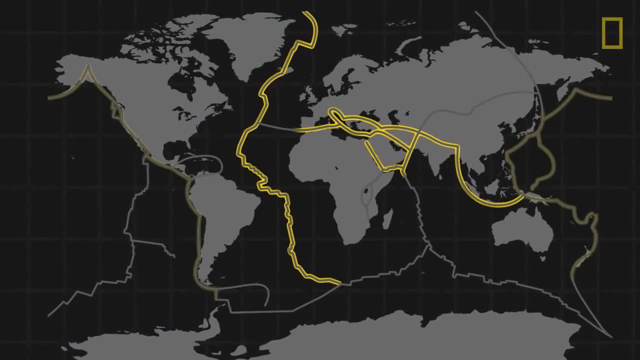 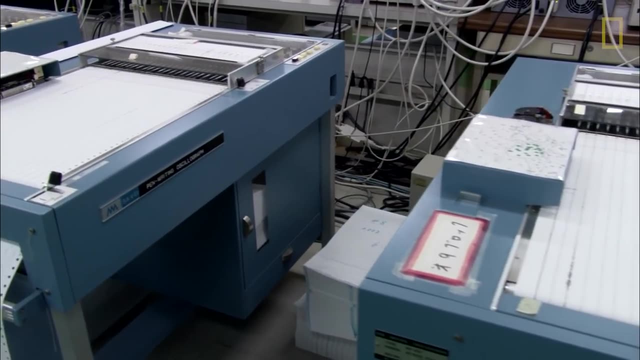 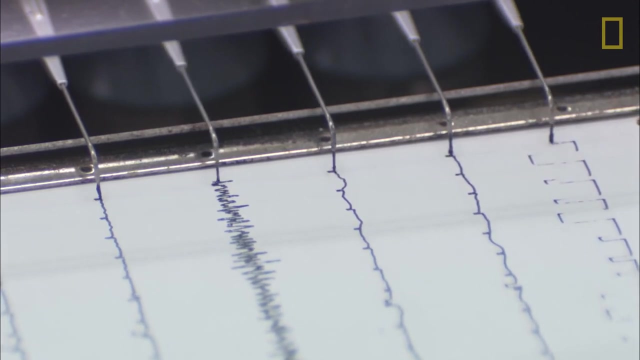 In fact, the world's most earthquake-prone regions are where the most geologically active plates meet. Earthquakes, or any seismic activity, are recorded by seismographs. When the ground shakes, seismographs oscillate, drawing a jagged line to reflect this movement. 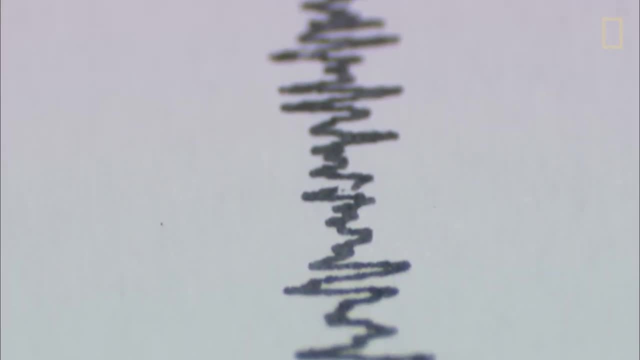 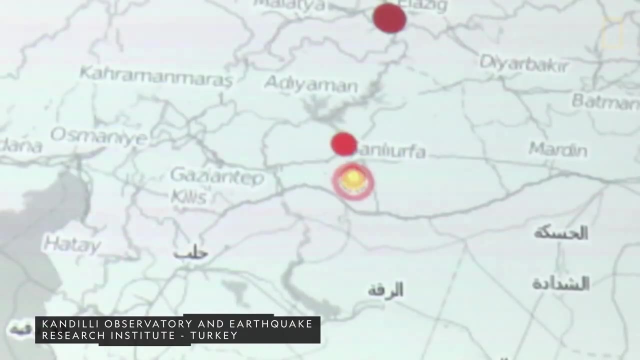 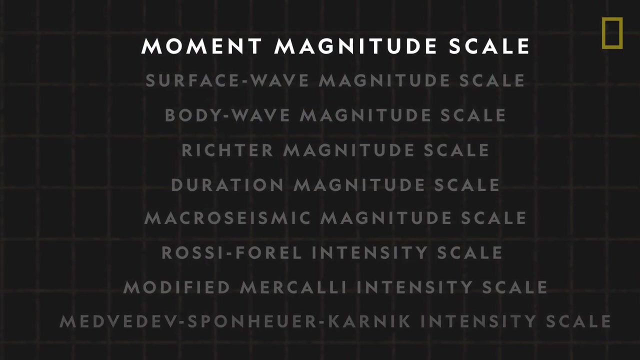 The more extreme the earthquake, the greater the height of the jagged line. These recorded motions are then used to measure the earthquake's strength or magnitude. While several scales of magnitude exist, the one seismologists prefer is the moment magnitude scale. 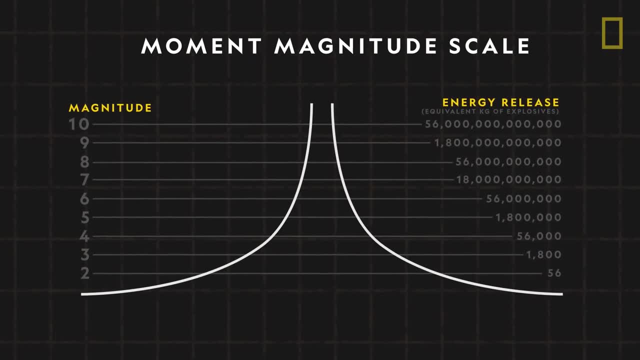 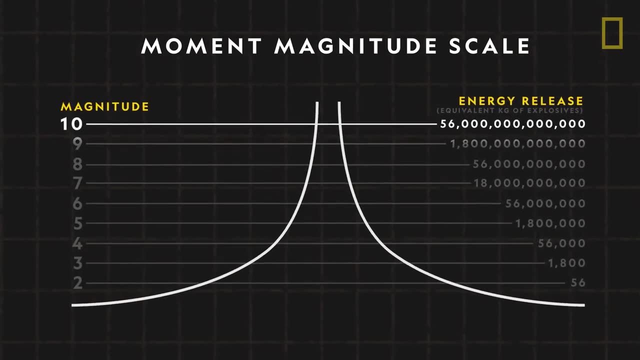 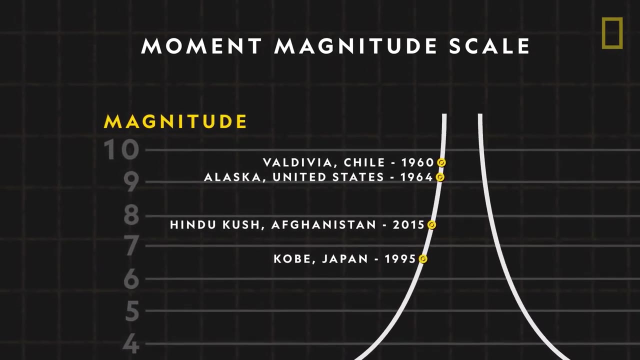 It has no upper limit and it measures earthquakes logarithmically. This means that each magnitude on its scale is ten times greater than the one before it. Unlike the now rarely used Richter scale, the moment magnitude scale can be applied globally and can measure quakes of the highest magnitudes. 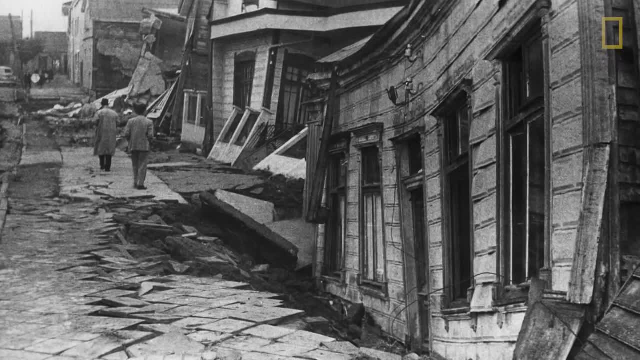 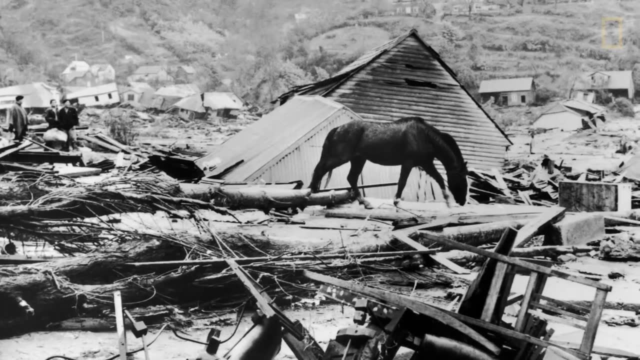 The largest recorded earthquake occurred near Valdivia, Chile, in 1960.. Nestled within the circum-Pacific belt, the Valdivia earthquake was the most powerful in a series of quakes that struck the region, measuring at a magnitude of about 9.5.. 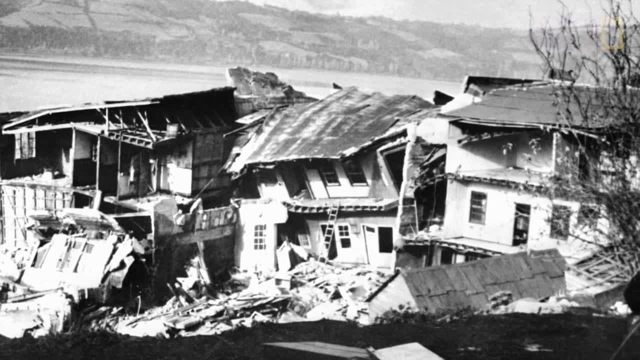 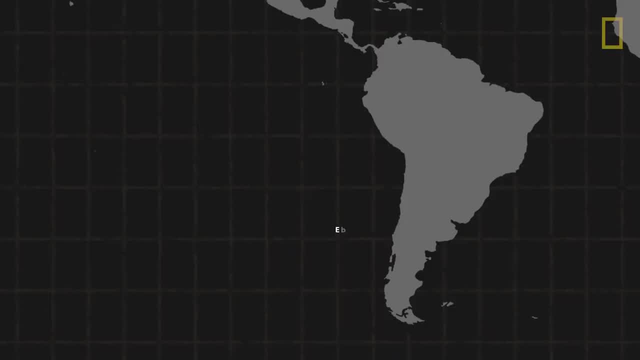 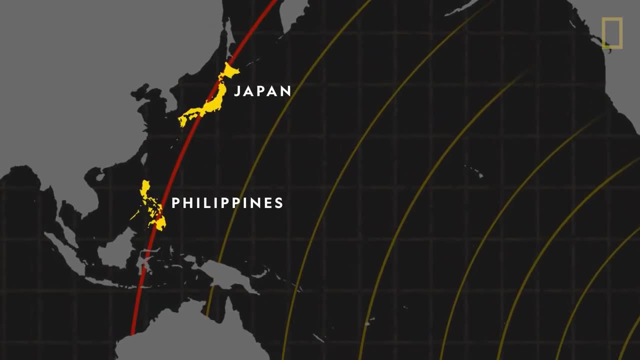 In addition to causing devastating tremors on land, the earthquake also generated a deadly tsunami reaching up to 80 feet high. The tsunami raced across the Pacific Ocean, hitting faraway countries like the Philippines and Japan. In fact, data from seismographs show that the shock waves emitted by the Valdivia earthquake 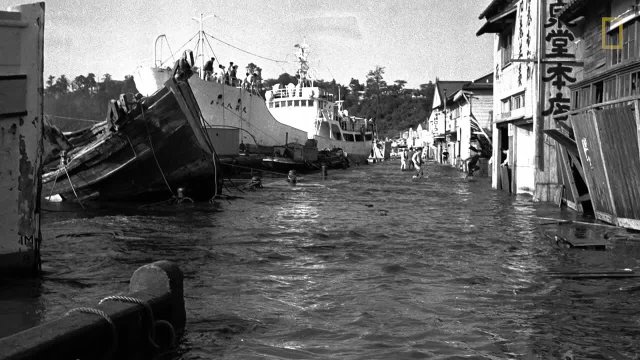 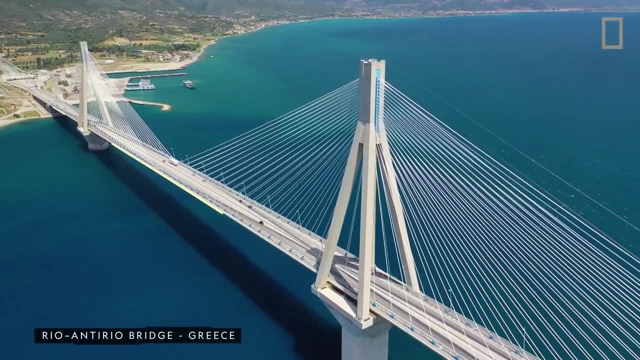 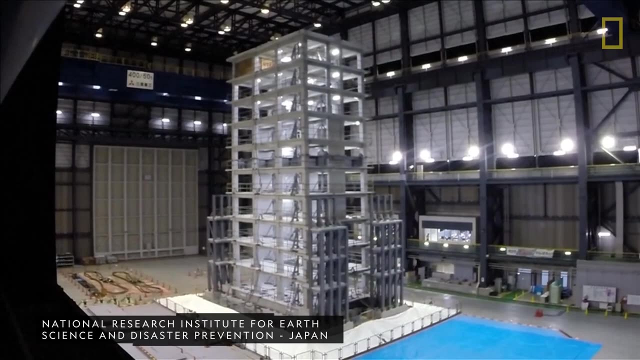 continued to shake the entire planet for days. Some earthquake-prone areas have adapted various ways to protect their communities. Buildings and bridges are designed to sway rather than break when an earthquake occurs. The public is educated on how to protect themselves during a seismic event.